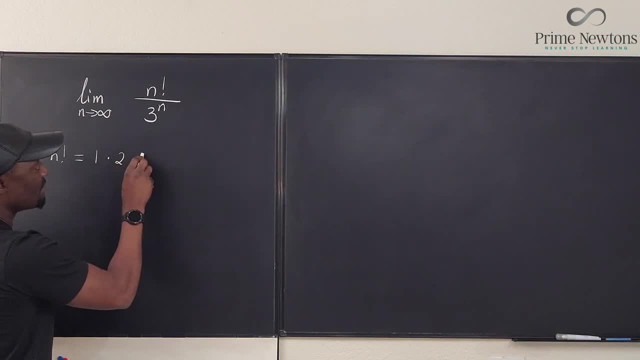 multiplied by 2, multiplied by 3, multiplied by- just keep going until you get to. let's say, you get to n minus 1, and then multiplied by n. We don't know what n is. Okay, now what about this? We know that 3 to the n is equal to 3 times, 3 times 3 times. well, we don't know how many We. 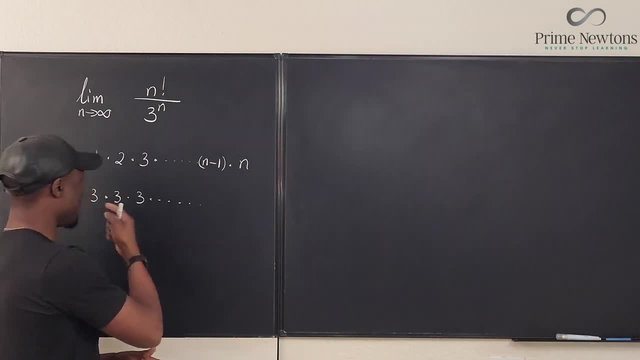 just, it just keeps going. There is no ending. It depends on how many 3s we need, depending on what n is, But whatever happens, we're going to have the same number of terms. Okay, so at the end of the day, we're going to have a 3 here, So you're going to have a 3 here. So you're going to have a. 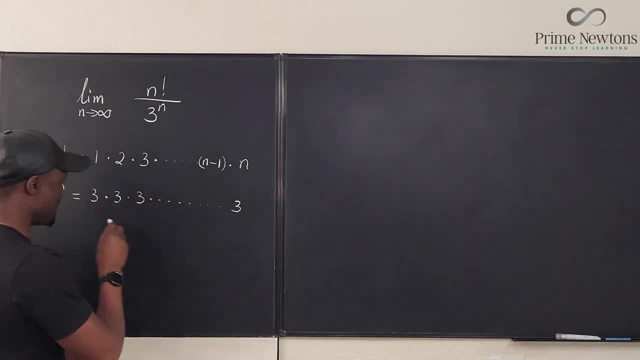 3 here. So you're going to have as many 3s, but the number of 3s you have is going to be n of them. So here there's going to be n 3s, That's 3 raised to power. n Multiply 3 by itself, n times. 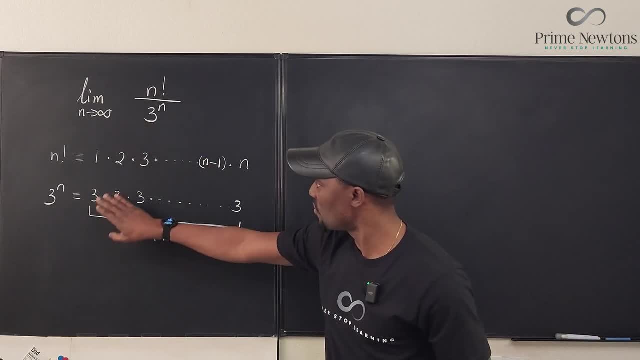 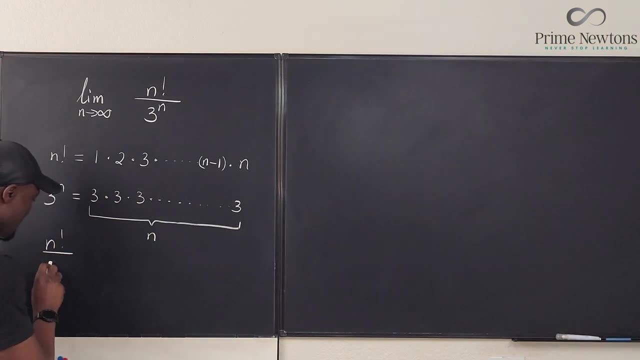 Okay, so let's rewrite this fraction then based on what we have shown here. It looks like our fraction here, n, factorial, divided by 3 to the n, can be written as 1 times 2 times 3 times. We're going to go like that until we get to n minus 1.. And then we have n times n And under. 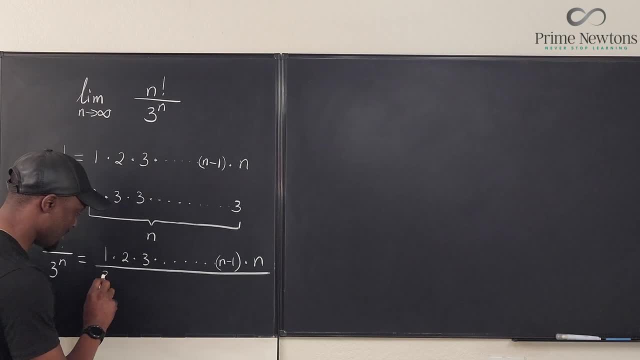 it because it's multiplication. we can write 3 times. 3 times 3 times, We get. here, we write 3.. Here we write 3.. Everything looks nice. And because it is multiplication, you see, I've 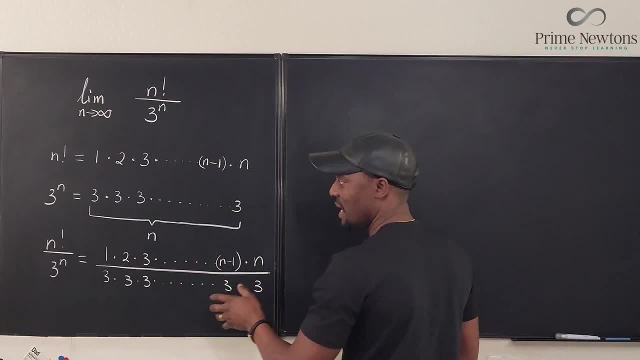 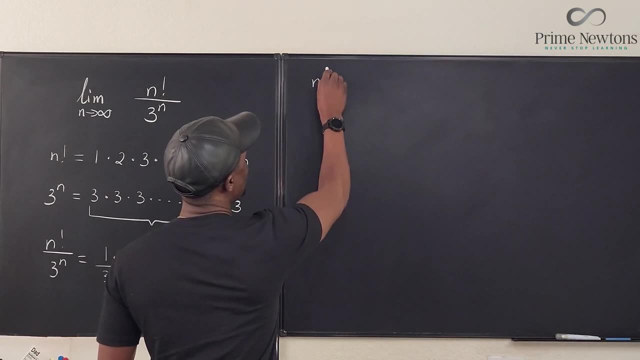 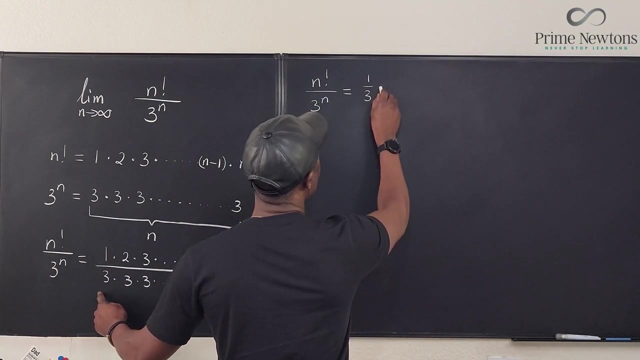 ignored the limit for now. Okay, because it's multiplication. you can actually split these into fractions, So we can say that n factorial divided by 3 to the n is the same thing as 1 over 3.. Nice Times. 2 over 3 times 3 over 3.. Nice Times, there's going to be another number. Let's try it. 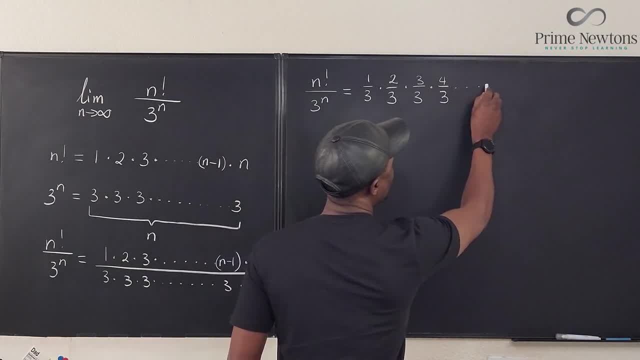 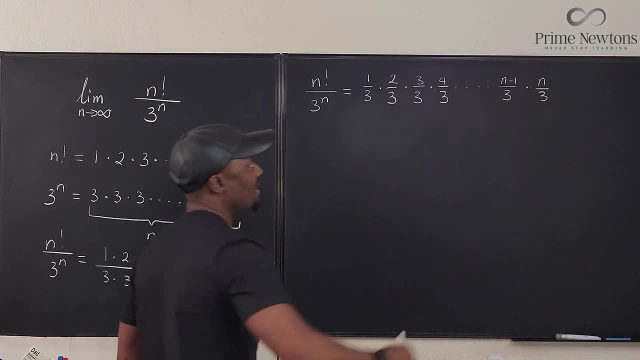 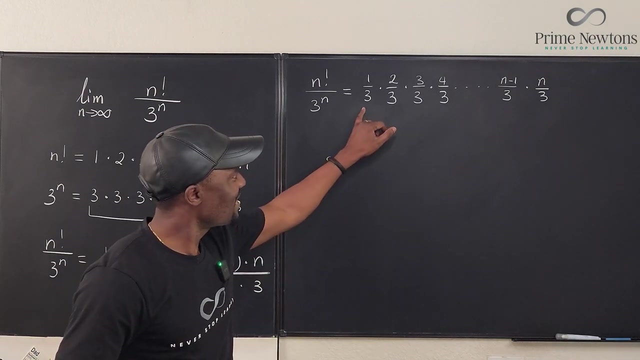 4 over 3.. Okay, top, top, top, top, We're going to have n minus 1 over 3 times n. That's what this is going to be. But I want you to pay attention to something. This is the same. 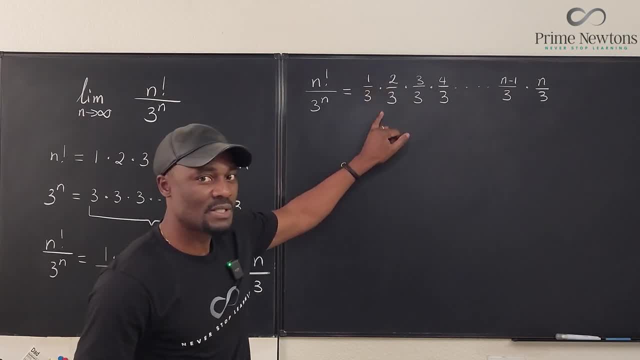 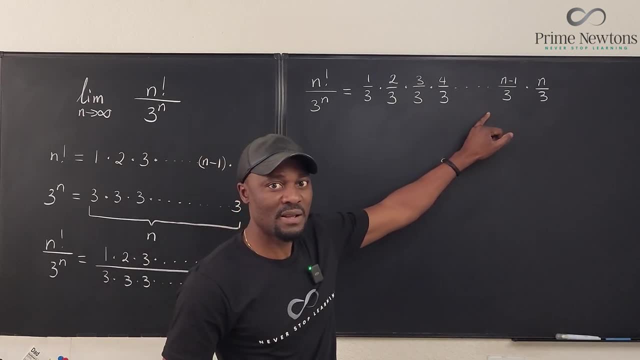 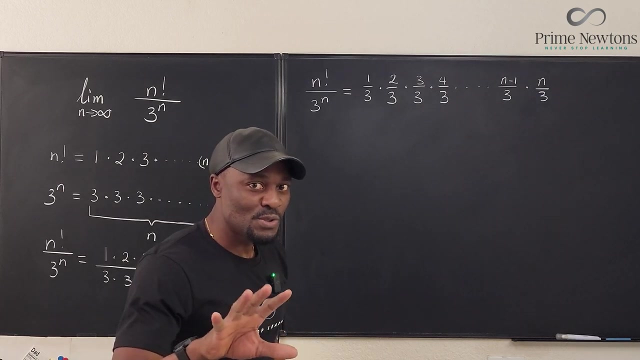 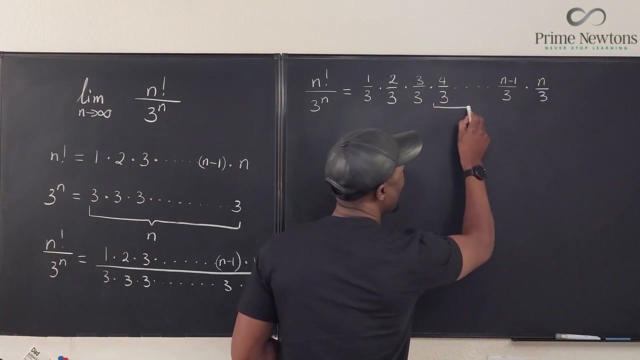 thing as 1 third times 2 thirds times 1.. After 1,, every single number here is bigger than 1, right, Okay. So if I choose to delete all of these, I delete everything here. Watch If I take everything here out of this multiplication. 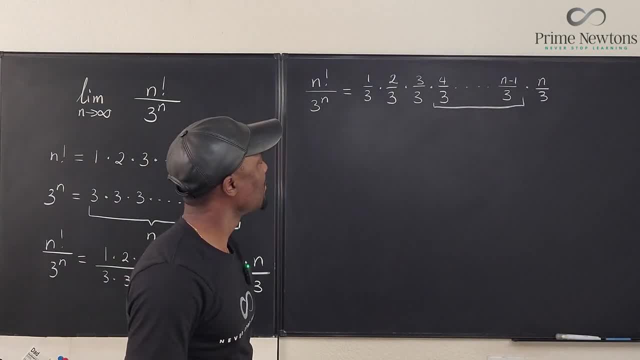 and I say you know what? I can claim that n factorial over 3 to the n must be greater than or at least equal to. listen must be greater than or equal to anything I write with any part of this missing, Because the full thing is all of this. 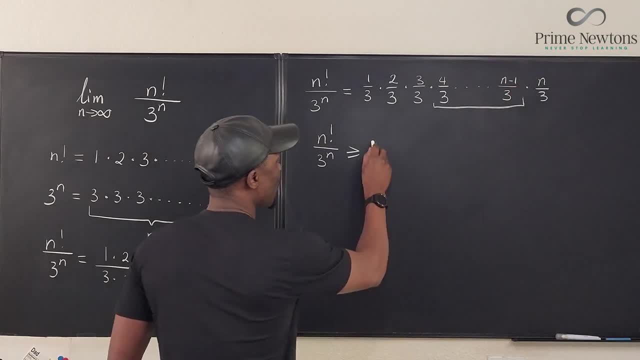 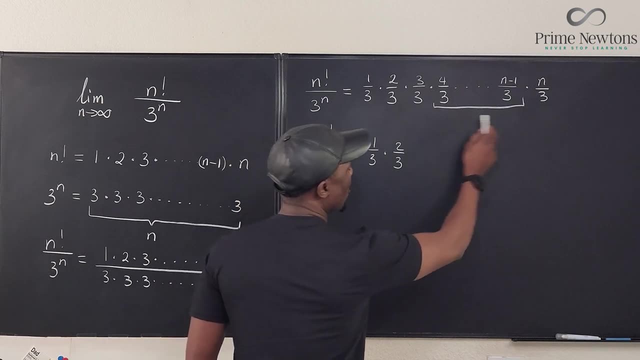 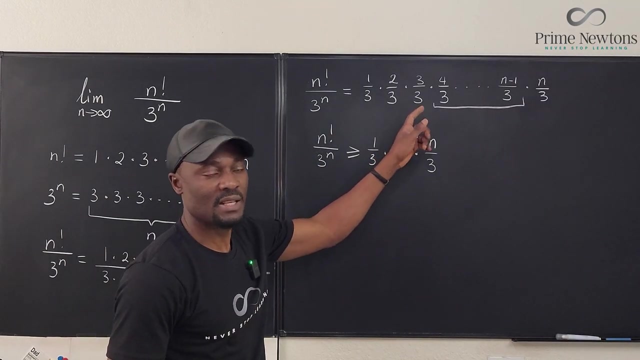 So I'm going to delete this part and just write 1 third times 2 thirds. Well, this is 1. It doesn't change anything, So I'm going to write times n over 3.. Because this is 1. There's no point writing it. 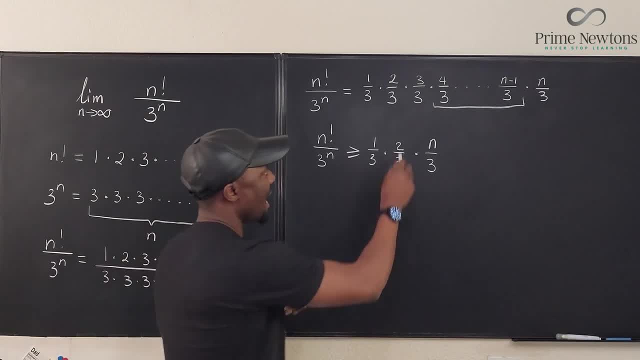 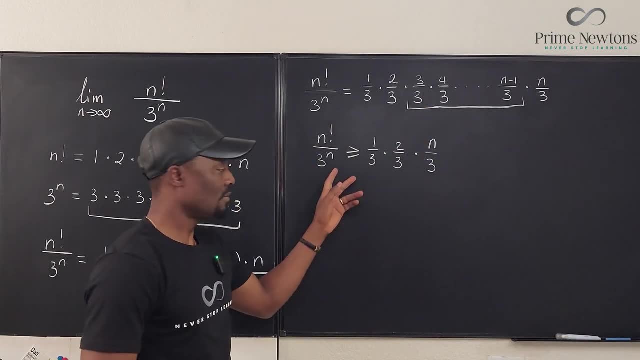 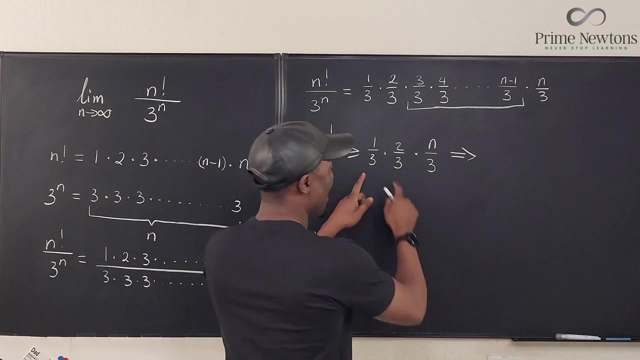 Look at that, So I can actually include this to what I'm deleting, because it doesn't make any difference. Is this true? Yes, it is true. So this implies that if I multiply this out, what would it give me? 2 over 27.. 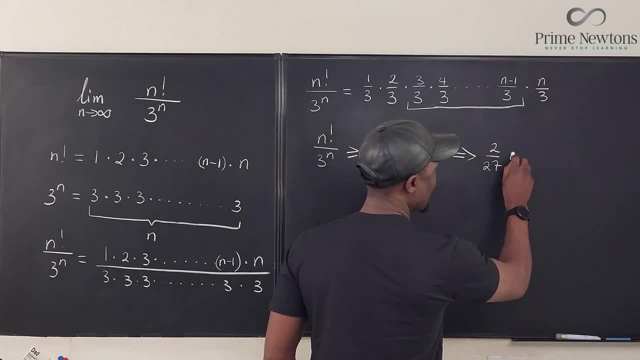 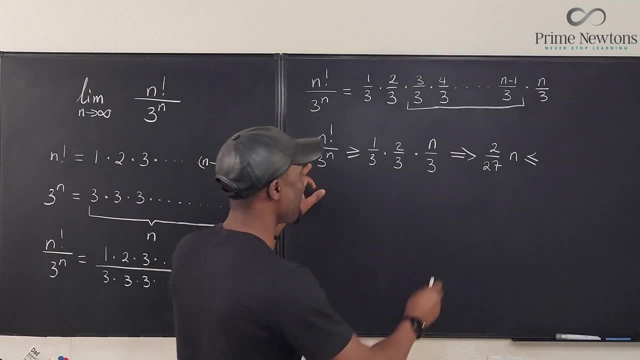 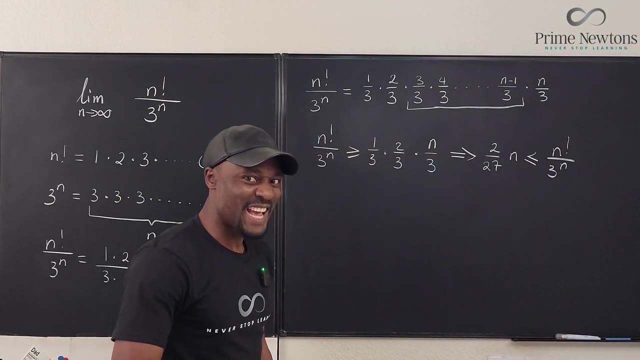 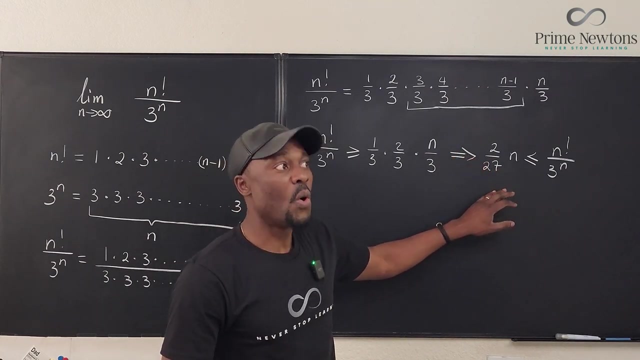 2 over 27n is definitely less than- or, in worst case scenario, it is equal to, n factorial over 3n. Now you can guess That's where I'm going with this. Whenever you have a function or, let's say, a sum, 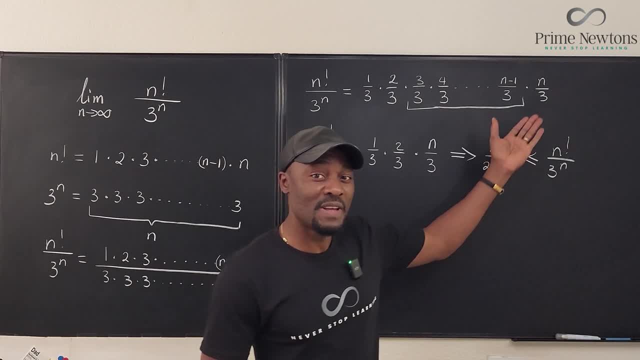 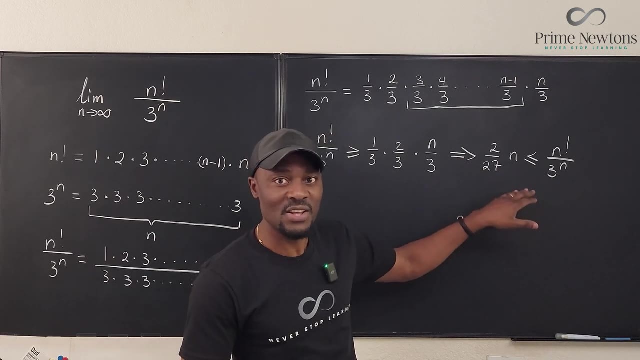 or anything that goes to infinity and it is less than another thing and it's under it. so I'm trying to show you the direct comparison method here of checking whether something converges or diverges. This is the test of the direct comparison test for divergence.